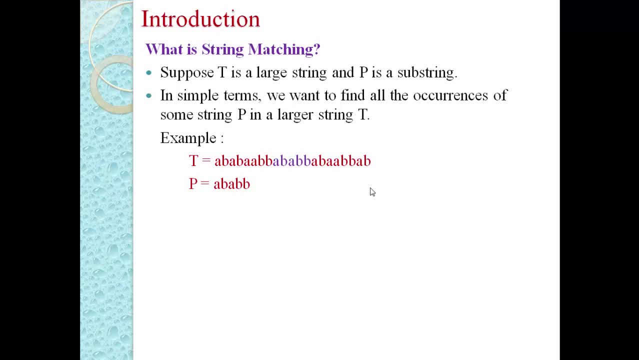 string capital T. So we have a certain algorithm to find whether the string is available in this large string or not. If multiple occurrence of the same pattern is available, then we can have a index number of every occurrence. So let us discuss the difference between the 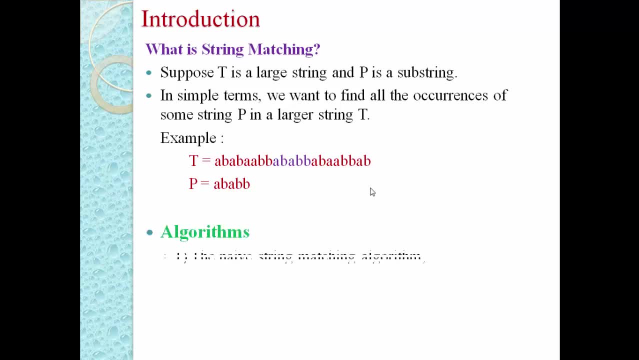 different algorithms. There are number of algorithms for string matching. First, one that is a very classic and brute force algorithm, that is, a new string matching algorithm. Second, the Rabin-Karp algorithm. Third, string matching with finite automata. And fourth, KMP algorithm. 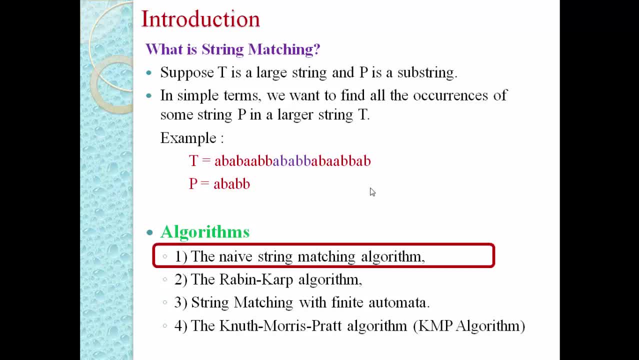 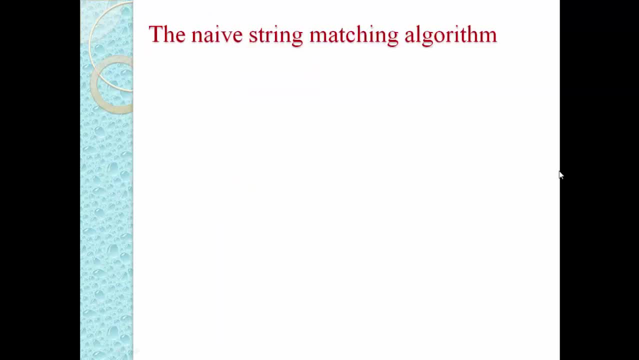 In our today's video, we will discuss our first classic algorithm, that is, a brute force algorithm, And this algorithm is known as KMP algorithm. So, as per the concept of a new string matching algorithm, match pattern string against input string, character by character. When there is a mismatch, shift the whole input string. 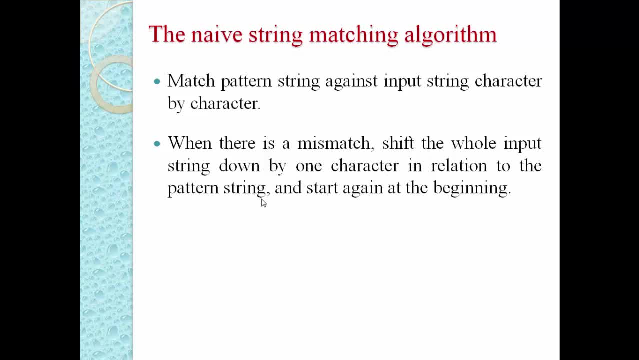 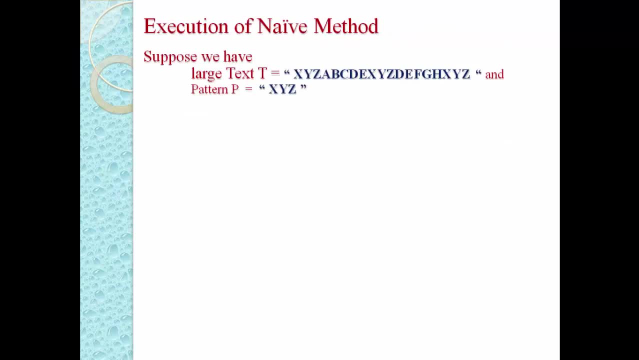 down by one character in relation to the pattern string and start again at the beginning. So just take one example so that you can easily understand the concept of new string matching. Suppose we have a one large text, capital T and these all are the different character. 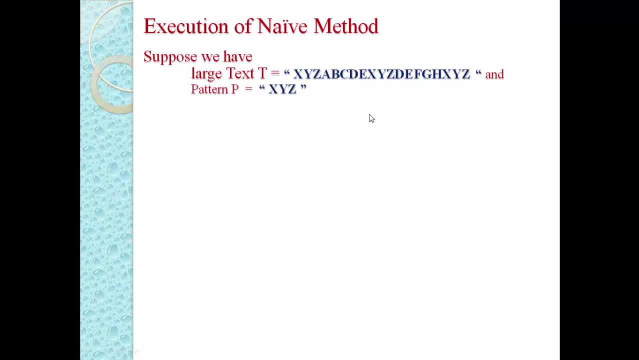 of our capital T string And another string that is capital P. this capital P is known as pattern string, which has a three character XYZ. Now our basic concept is we have to match this string XYZ, or we can say we have to match pattern with all the character of our large 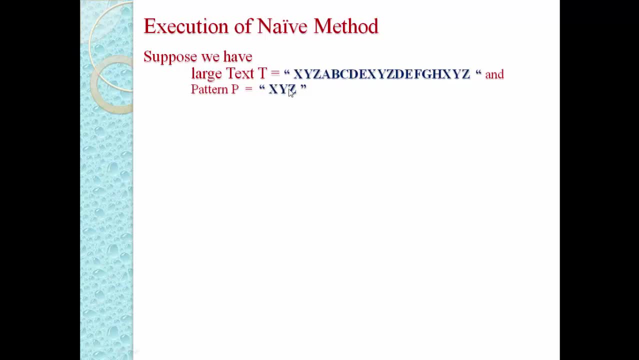 text capital T And we have to identify whether this pattern is available in this string or not. Once we get pattern inside the text capital T, then we have to return index number. This large string, capital T, may have multiple occurrence of the pattern capital P And for every occurrence. 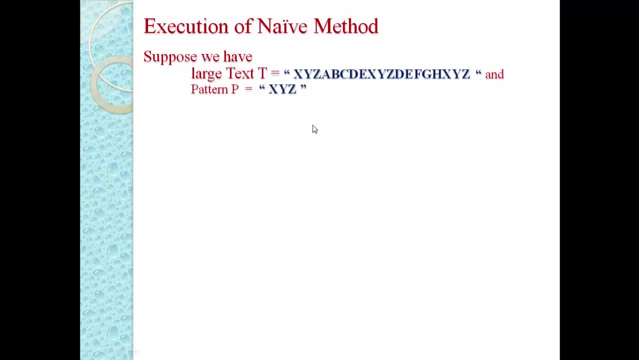 we have to return index number. So let us write this both: the string with index number. This is our first string that is capital T and it is a large string. We have written with this index number because we have stored this whole string inside one array And array. 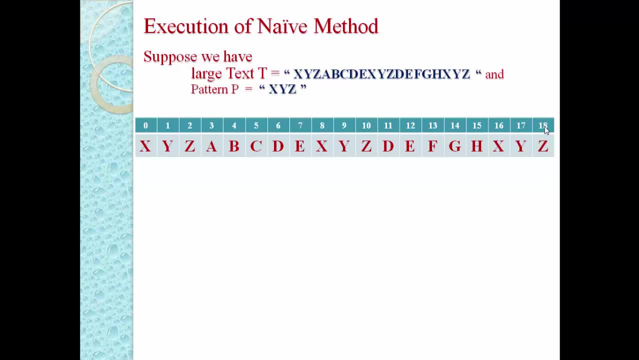 starting from the zero, So total 19 characters are there in our large string, capital T, And we are starting from zero to 18.. Same way, another array, that is capital P, has a three different characters and starting from zero to two. So three characters are there and 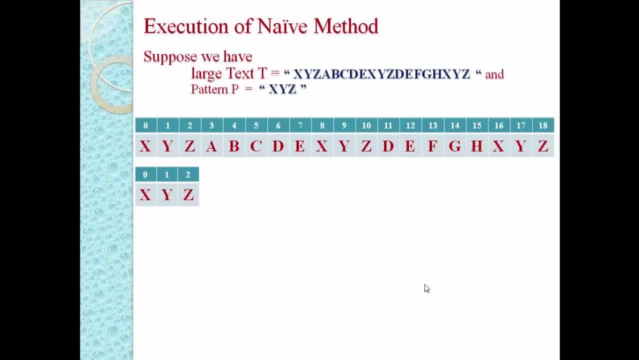 we have to write inside our pattern capital P, And here we will display output, And it is nothing but index of every occurrence. So let us start our new method to find every occurrence of our pattern inside our large text, capital T, So, as per the concept of new 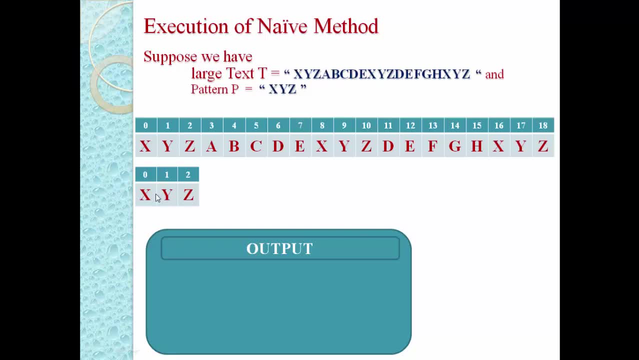 string matching algorithm. we have to compare all the character of pattern with our large text capital T. In our pattern we have only three characters, So first three characters we will compare with first three characters of our large text capital T. So x will compare with x Matching. 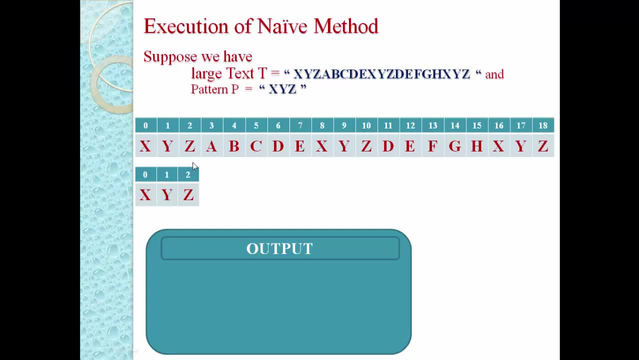 is found, Y will compare with y, Matching is found And z will compare with z. So this, all the characters were found inside our large text capital T. It means that string, or we can say the pattern, is available inside the large text capital T, So we have to just write. 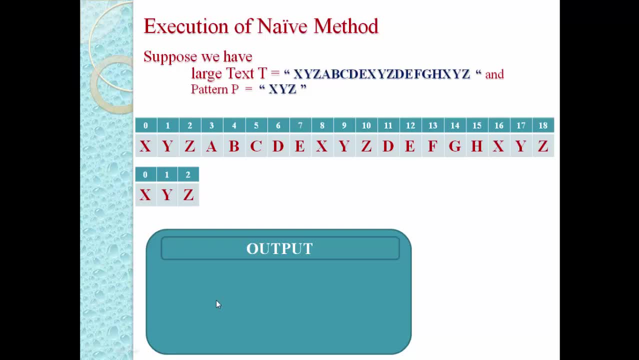 first occurrence of our string. So pattern found at index zero. It means that our first occurrence of pattern inside the large text, capital T, is from index number zero. There may be a multiple occurrence of pattern inside the text So that we have to check another, all the occurrence, And for 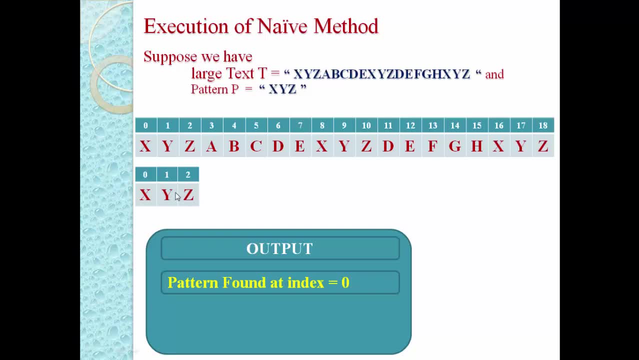 that we have to just shift our pattern by one. Once we shift our pattern by one, We can see that we have two patterns inside our large text, capital T. So after we shift our pattern by one, Then again we have to compare the character of pattern with the character of text. So we have to compare our second character. 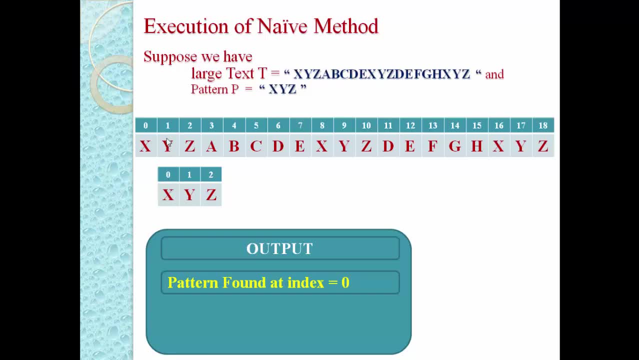 of our text with first character of pattern. So here it is y and here it is x. It means that matching is not found. So we have to again shift our pattern by one. So once we shift then we have to check, We have to compare third character of text with first character. 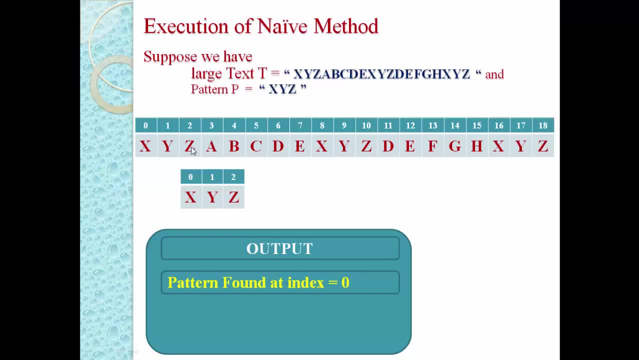 character of pattern, whether matching is found or not. here it is z and here it is x, so matching is not found. so again, we have to perform shift operation. once you perform shift operation, then we have to compare character a with character x. so matching is not found, so again we have to. 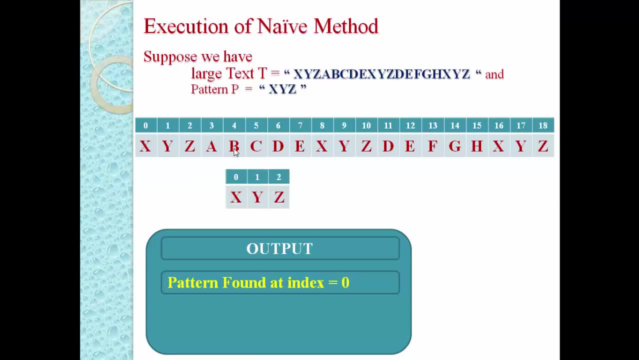 perform shift operation. now, again, we have to check whether b is match with capital x or not. so again, matching is not found, so that we have to perform shift operation. same way, we have to perform shift operation one by one. so now, when we reach here on index number eight, at that time when 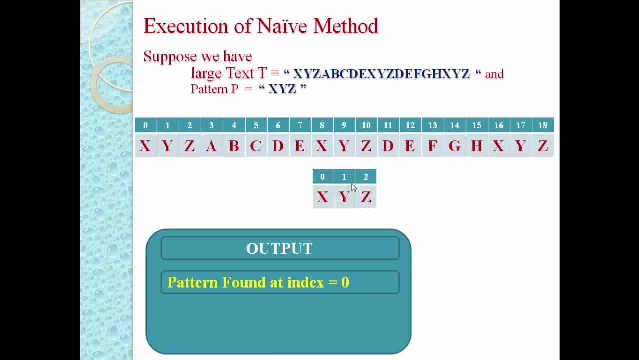 we compare x with x, matching is found. y is y with y, then matching is found. and z with z, matching is found. it means that this second occurrence is available at index number eight. so pattern found at index number eight. so there may be a chance that there will be another. 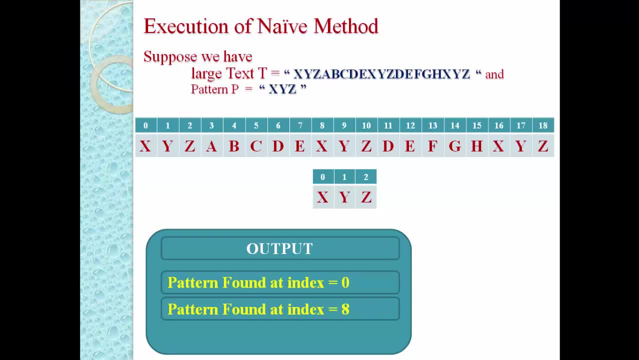 occurrence of pattern inside the text. so we have to shift again our pattern by one. so shift our pattern by one and compare with this character of text. so y. compare with x. no matching is found, so again perform shift operation. compare z with x. matching is not found, so perform shift. 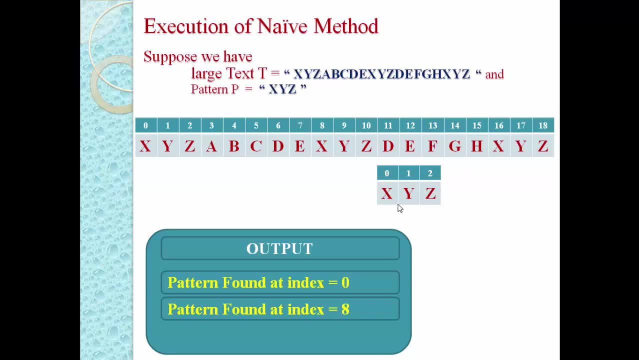 operation. compare d with x: matching is not found, so perform shift operation. compare e with x: no matching, so again perform shift operation. compare f with x: no matching, so perform shift operation. same way: check g with x: no matching is found, so perform shift operation. h with x: no matching is found. 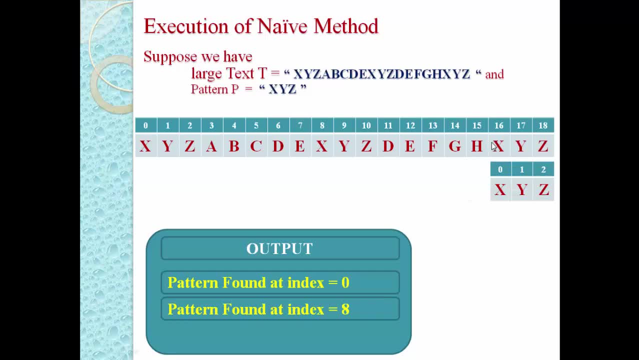 so perform shift operation. now: x: compare x with x, so matching is found. so second character: we need to compare y with y, matching is found. z with z, matching is found. it means that third occurrence of our pattern is on index number 16. so pattern is found at index number 16. so there are three. 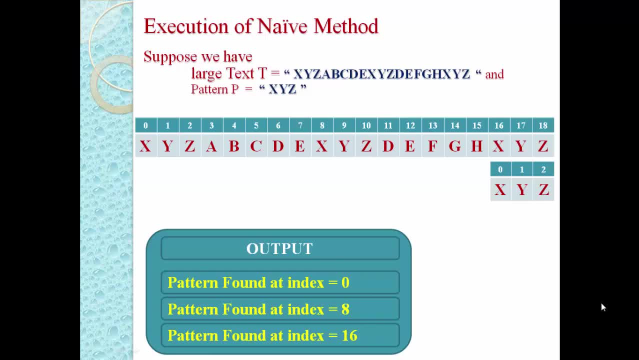 occurrence of our pattern inside our large text capital t. first occurrence at index number zero, second occurrence at index number eight and third occurrence at index number 16. now when we start to write the algorithm, then first step is we need to identify the length of our large text capital t and length of our pattern. so here the length of. 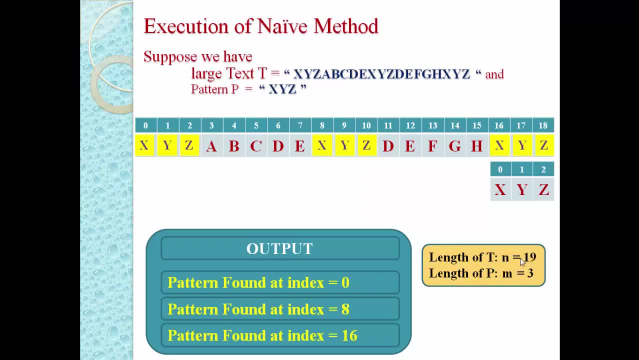 our large text, capital t is equal to 19 and the length of pattern is equal to three. suppose the length of capital t is known as small n and is equal to 19, and the length of our pattern p is, for example, known as m and m is equal to three. now we need to check how many times we 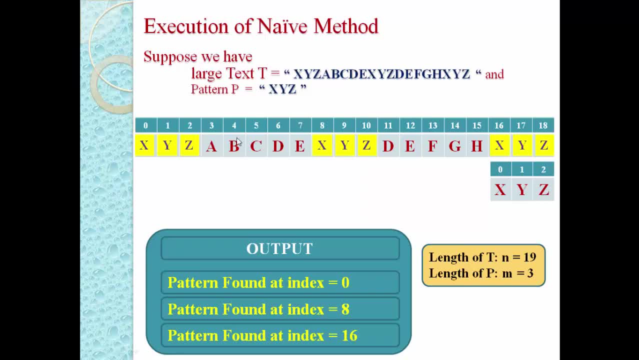 have to perform shift operation. we have started from zero and up to the 16, so total 16 shift operation we need to perform right. so how we can get 16? so here we can perform shift operation. like a: 19 minus 3 is equal to 16, so n minus m shift operation is required. and after every shift 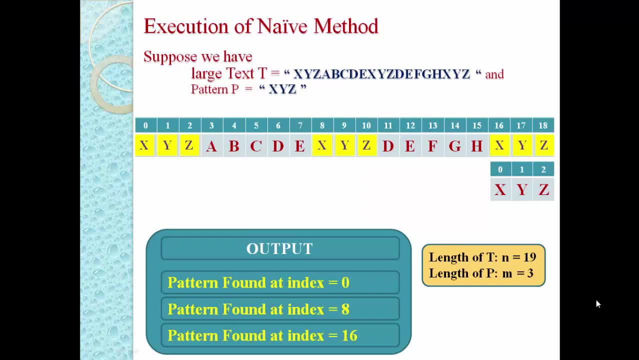 operation we have to perform comparison, comparison of pattern with the text. so maximum how many comparisons required it is depends on the size of our pattern. here three characters are there. then after every shift operation there will be maximum three comparison of pattern. so we have to perform pattern with the text. so here two different loop is required. first loop, that is the outer loop, to 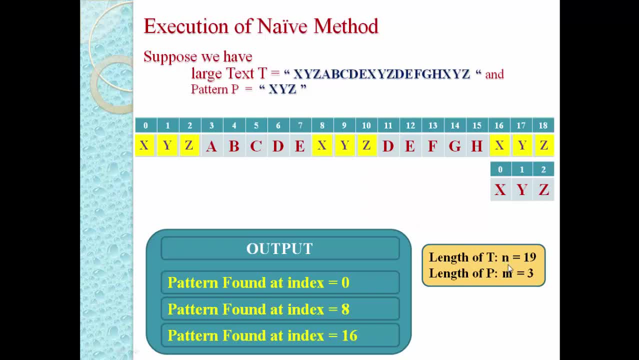 perform shift operation and this loop will be executed n minus m time. so outer loop will be executed n minus m time and one another inner loop is required, and this inner loop basically used to perform comparison of all the character of pattern with the text and maximum m. 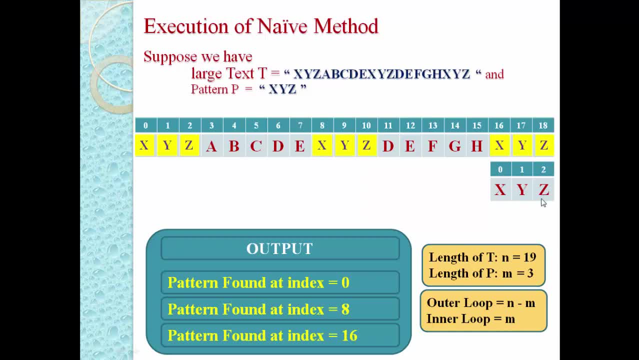 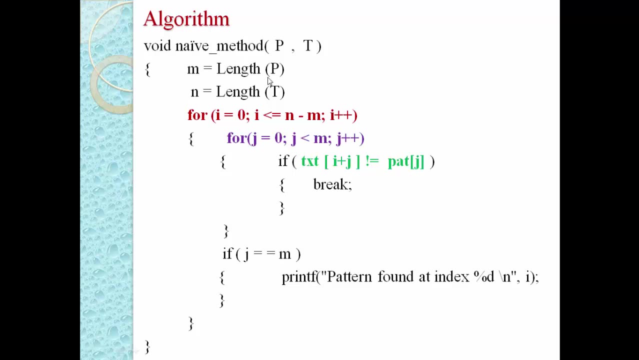 comparison is required because the length of our pattern is m, so total m time this inner loop will be executed. so let us see the pseudo code of our new method. as per the pseudo code of our new method, first identify the length of pattern, then length of text. as we discuss, we will have a two loop: one,